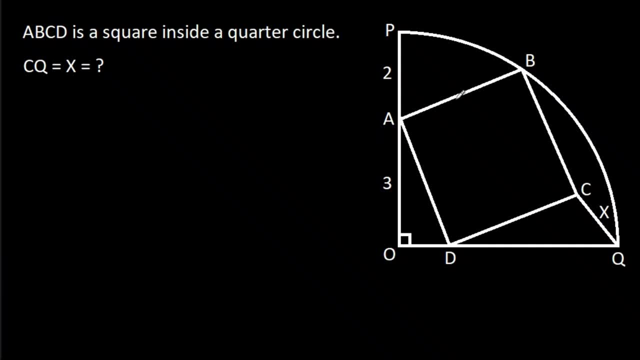 In this video we have been given that ABCD is a square inside a quarter circle and PA is 2, AO is 3 and CQ is X, Then we have to find X. So we have PA is 2 and from point B, if we make a perpendicular on PO, 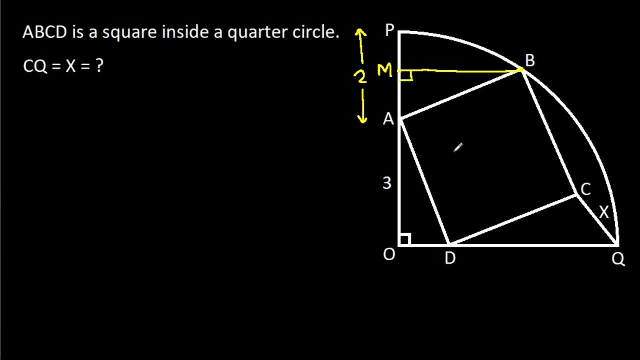 suppose this point is M, and from point C, if we make a perpendicular on OQ- suppose this point is N- then if this angle is ANPHA, then this angle is 90 degree. So this angle it will be 90 degree minus ANPHA. 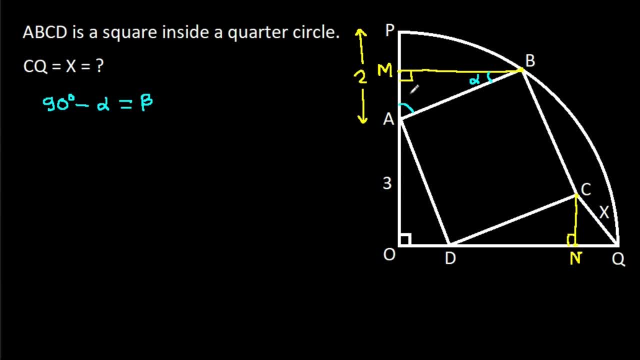 Suppose BETA, So it will be BETA and we know that ABCD is a square. So this angle, it will be 90 degree. So this angle, it will be 90-beta and that will be ANPHA, and this angle is 90-degree. 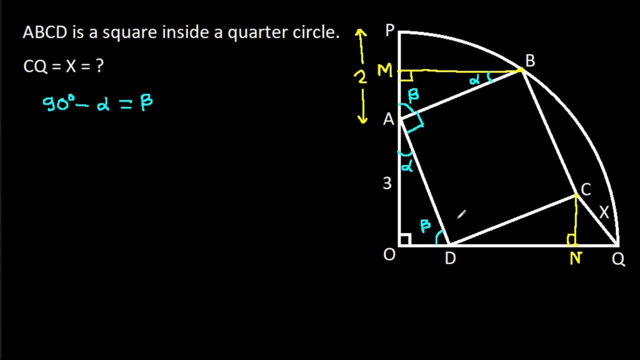 so this angle, it will be beta. and this angle, it will be 90 degree. so this angle, it will be alpha. and again, this angle is 90 degree, so this angle, it will be beta. so inter angle BMA, terangle AOD and terangle DNC, all these three angles are equal. 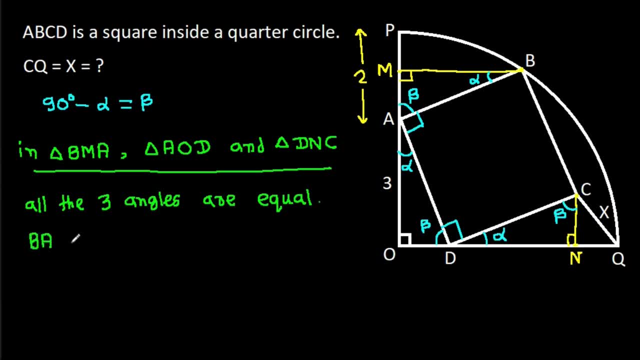 and also BA. it will be equal to AD, it will be equal to DC, because ABCD is a square. hence, terangle BMA, it will be congruent to terangle AOD, it will be congruent to terangle DNC and. 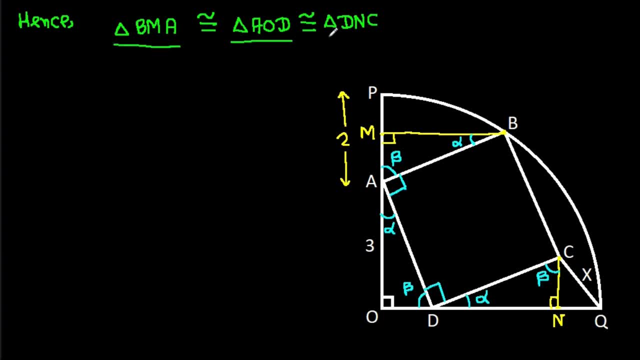 these three terangles are congruent. so BM it will be equal to AO it will be equal to DN and AO it is three. so BM it will be three and DN it will be equal to three. so EM it will be 3 and 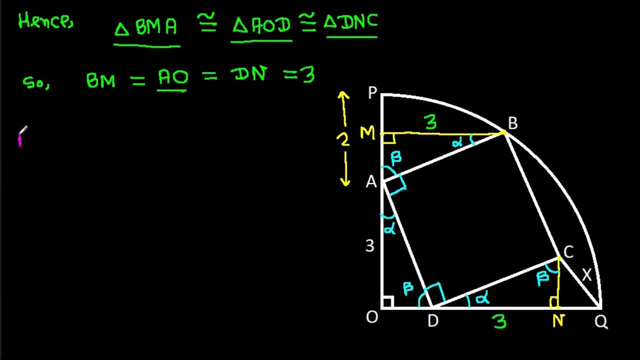 DO, it will be three and EI and instead AD, and then rad of del people will be there and will be equal to DLIL. it will be equal to 109.. So, in every angle, this angle will be union of ETB and 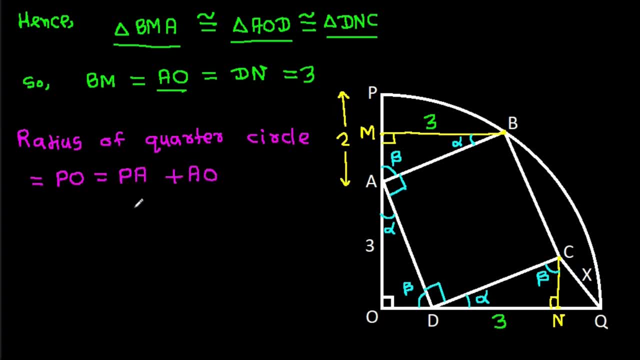 the radius of this quanta, Soon after d� will be reversed and it will be的人. 2 plus AO is 3, that is 5. And if we join OB, then OB it is also radius of quarter circle. 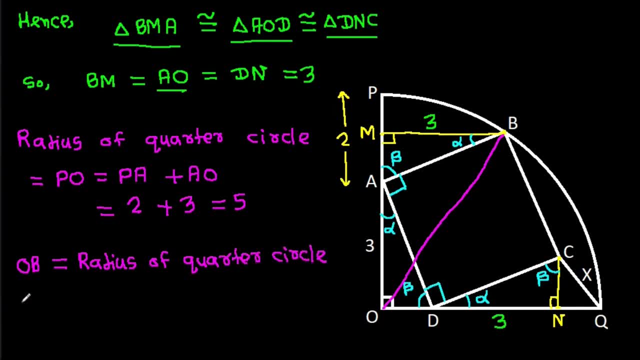 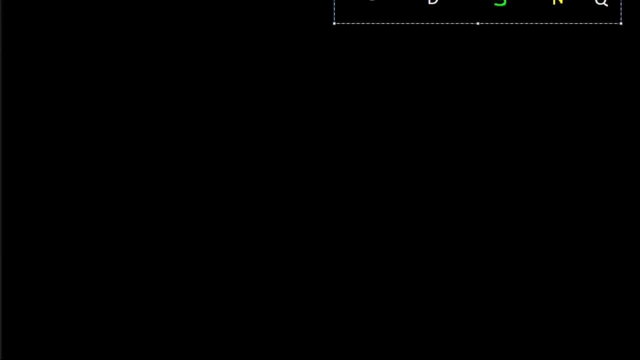 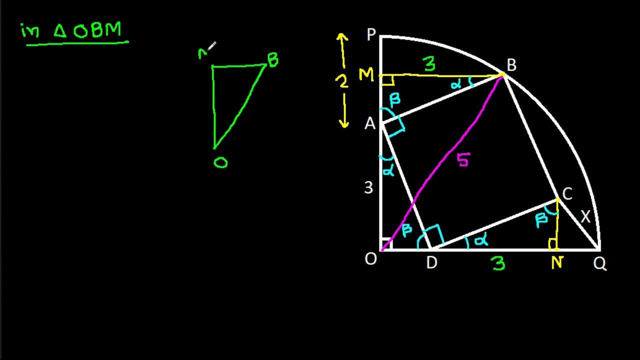 So OB it will be 5.. OB is 5.. And now inter angle OB It is OBM. this angle is 90 degree, OB is 5, BM is 3 and OB square it will be equal to OM square plus BM square by Pythagoras theorem. 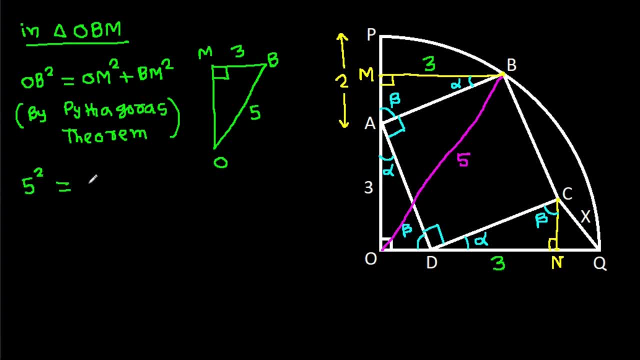 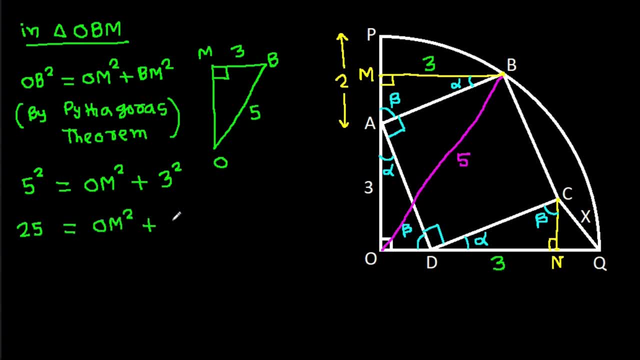 It is 5.. It is 5.. It is 5.. It is OM square plus 9.. So OM square it will be 25 minus 9, that will be 16.. So OM, it will be root 16, that will be 4.. 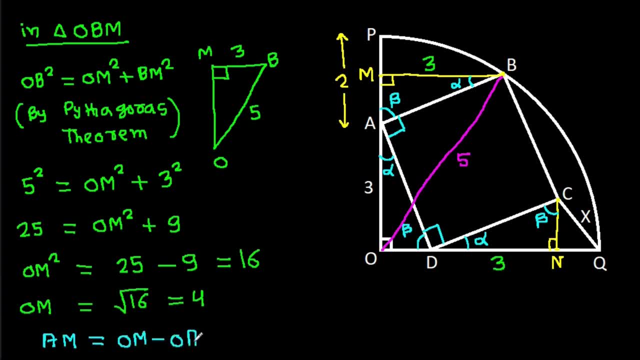 And AM it will be root 16,, that will be 4.. So it will be OM minus OA, and OM is 4 minus OA is 3, that will be 1.. So AM, it will be 1.. 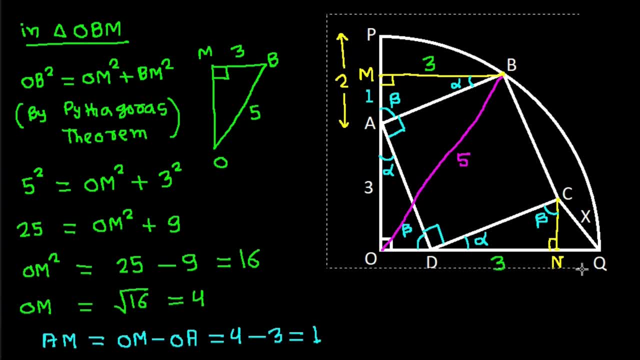 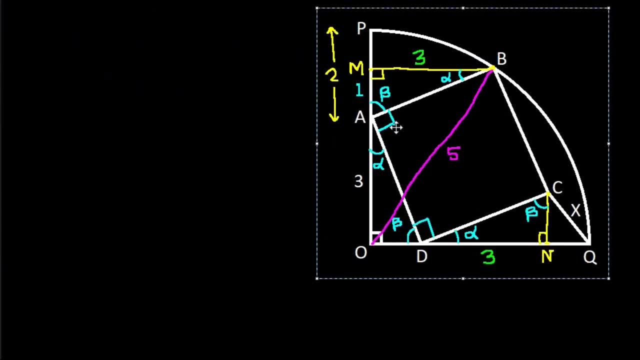 So AM it will be 1 and So AM it will be 1. and Now we know that triangle BMA it is congruent to triangle AOD and it is congruent to triangle DNC. So MA it will be equal to OD, it will be equal to NC. 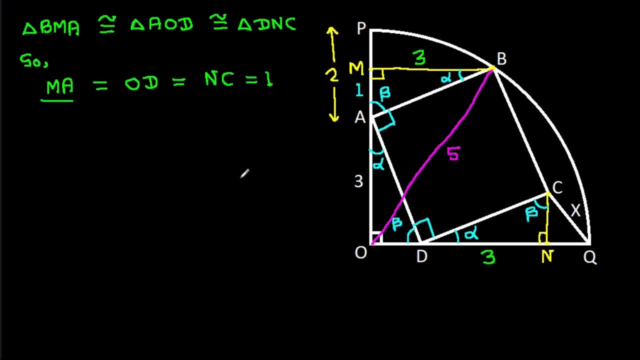 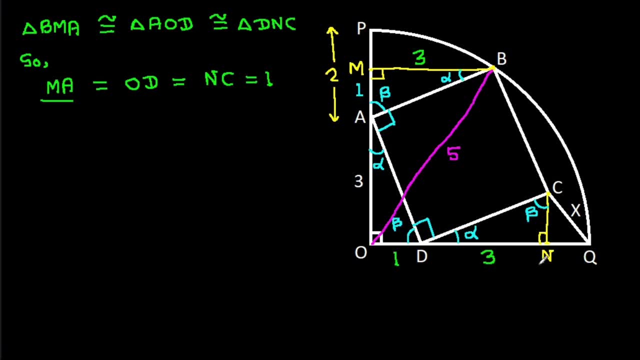 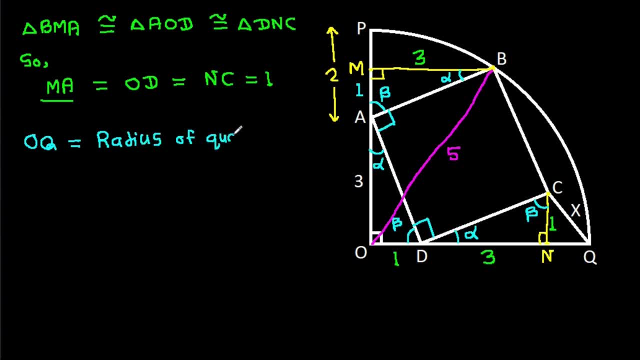 So OD it will be 3 and NC it will be radius of quarter circle. So OQ it will be 5 and OQ it is OD plus DN plus NQ it is 5 and OD is 1 plus DN is.